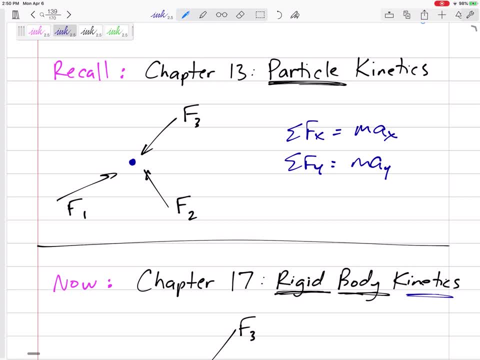 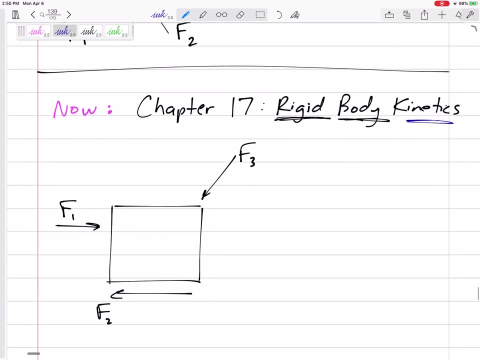 Maybe it was 3D: summing the forces in Z equals MAZ. Maybe we were summing the forces in normal, equals MA normal, summing the forces in tangential, MA tangential. But we were all just assuming that all of the forces were acting through the same point, But really they may not be, And so now that we have rigid bodies, all of these forces may not be acting through the center of gravity G, And so how will that change things? 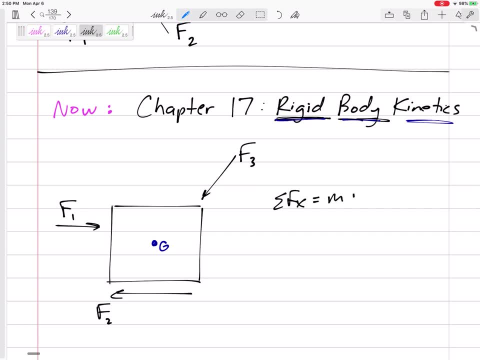 We will still sum the forces In X equals M- AX. sum of the forces in the Y direction equals M- AY. For 3D, we'll sum the forces in the Z equals MAZ. Many times those accelerations might be zero, But now we have moments, And so now we can sum the moments. You know what sum of the moments is equal to. In statics, sum of the moments is equal to zero. In many of these problems, sum of the moments will still be equal to zero. 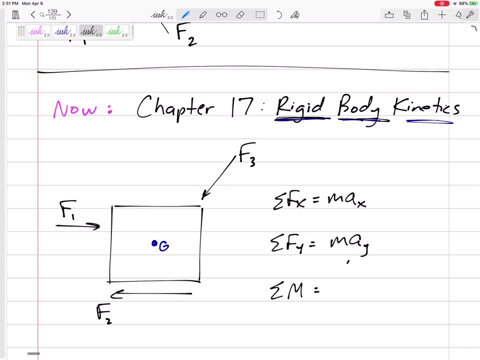 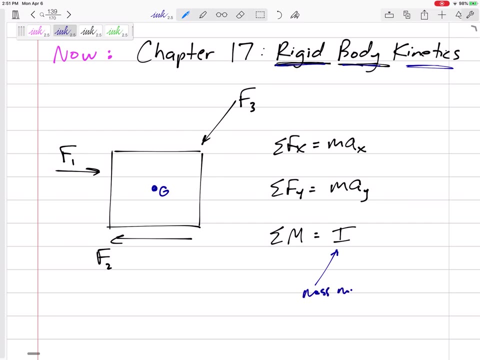 So we can sum the moments, But sum of the moments instead of mass times. acceleration instead of mass. we have I, We have I, which is the mass moment of inertia. So this I will be the mass moment of inertia. It's almost the angular equivalent of mass. It's a measure of an object's resistance to rotation. 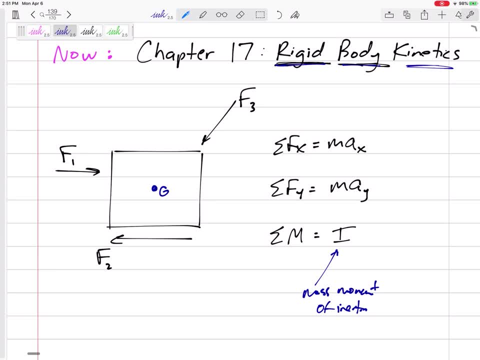 It's a measure of an object's amount, of how much mass is away from the center of rotation and how far it is away from the center of rotation. If you were in my statics class, we really compared mass moment of inertia with area moment of inertia, not to be confused with those two. But anyway, sum of the moments equals I, And instead of acceleration we've got alpha, the angular acceleration. 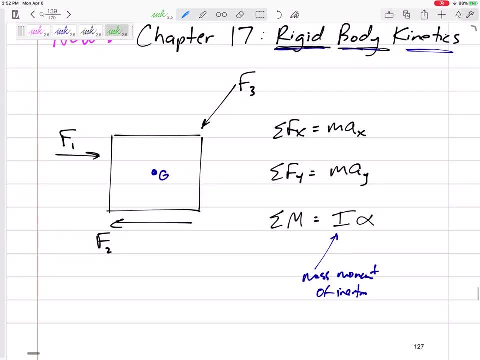 Okay, But one thing: we need to be careful with these points because this acceleration, if this is rotating, point G might have a different acceleration than point A or point B. So this is the acceleration of the center of gravity G. These are the accelerations of the center of gravity And this is the sum of the moment about the center of gravity. If we sum the moments about the center of gravity G, it's equal to I about G alpha. 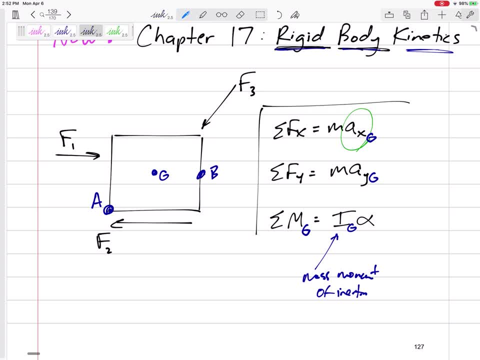 It's equal to I. about G- alpha. Now we'll talk about some exceptions to this equation, or some not exceptions, but if we sum the moments at a different point it may not be equal to I, G, alpha, But in general, sum of the moments is equal to I- alpha. But be careful about the points that we're looking at. So these are the accelerations of the center of gravity. 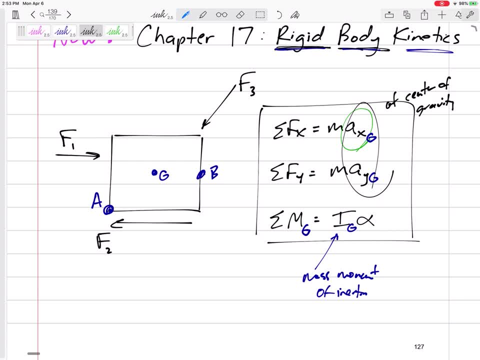 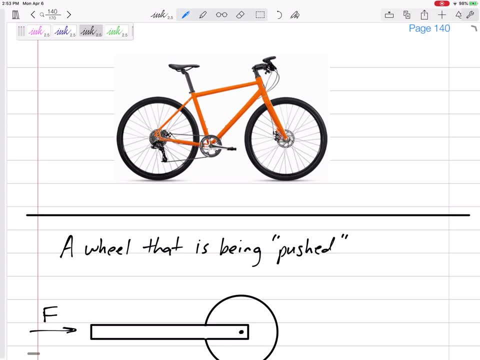 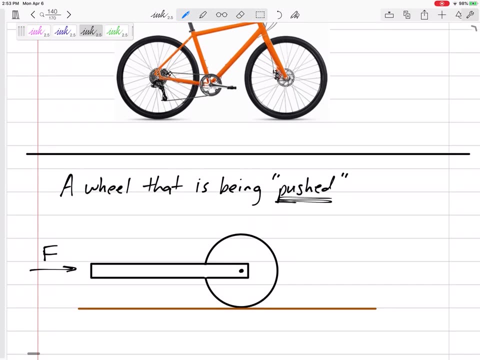 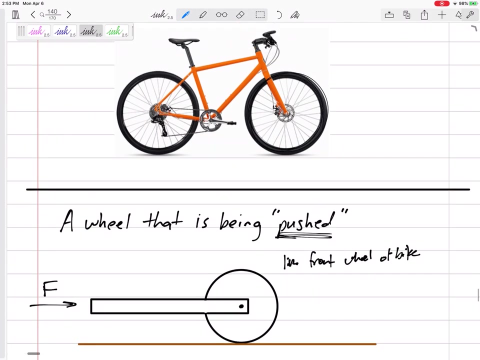 Accelerations of the center of gravity. Okay Now, one thing that I like to talk about we might see in some of these problems are wheels that are rolling, And many times wheels are either being pushed like the front wheel, the front wheel of a bike, right. This wheel right here is being pushed from that point right. 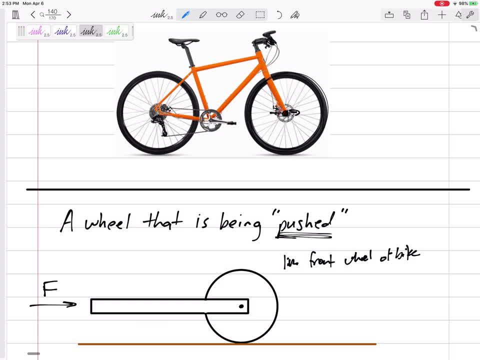 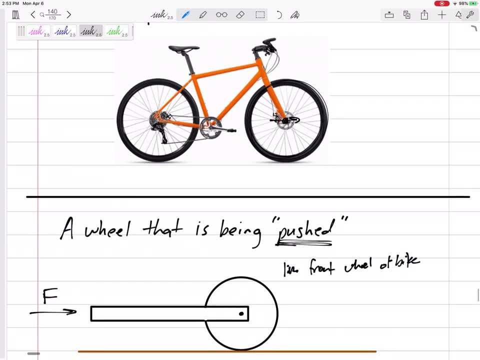 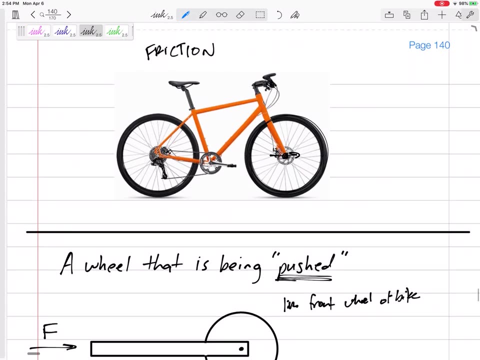 There. That point is pushing it forward, And so I want to talk about friction. Let's talk about friction on wheels that are being pushed, or wheels that are being turned. You might think that the force of friction- I don't know what direction do you think the force of friction is on these wheels right at this point down here? You might think they're backwards, forwards. 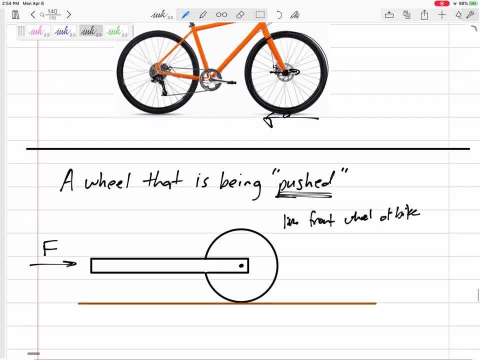 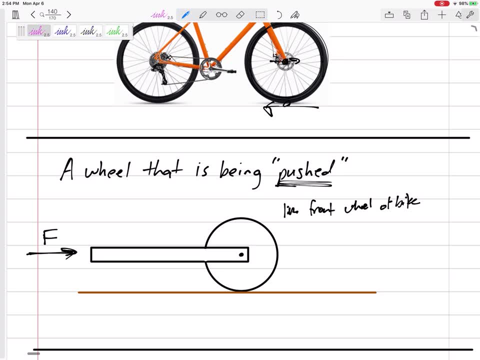 different than the back wheel. The front wheel is being pushed, Wheels that are being pushed with a force F. right here I've got a force of friction down here, but should I put the force of friction this way? Should I put the force of friction the other way? Friction opposes. 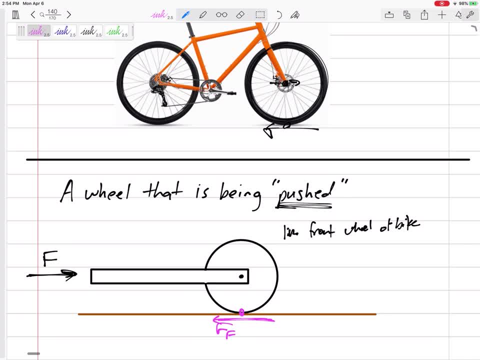 relative motion opposes impending relative motion. There's zero. if this wheel is rolling without slipping, That velocity is zero. This is static and so it's not really going left or right, but it opposes impending relative motion. but the way that I would think about this is: 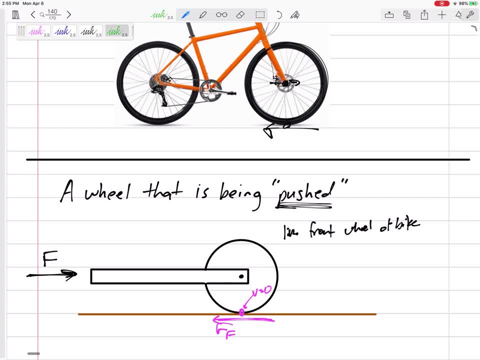 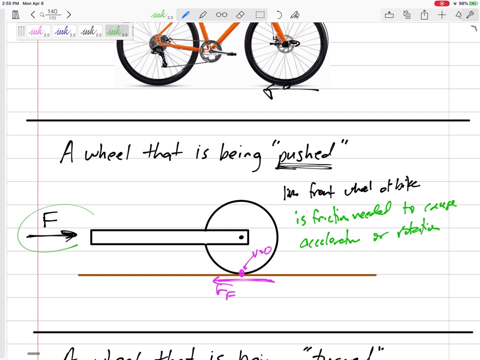 is friction needed to cause acceleration or rotation. Sometimes this helps me. If there was no friction, then this force right here would accelerate it forward, but there would be nothing that would cause any rotation. In this case, friction is needed for the rotation. If there was no friction, 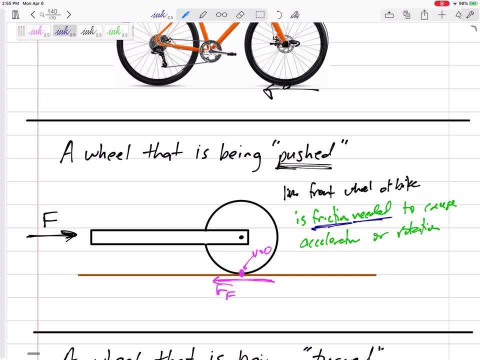 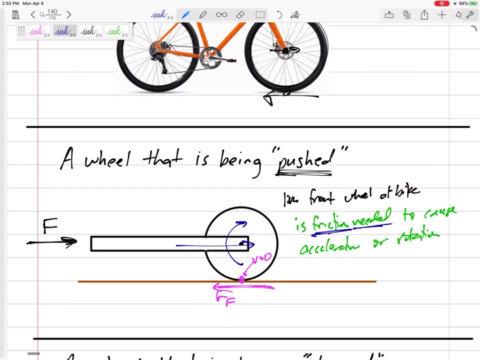 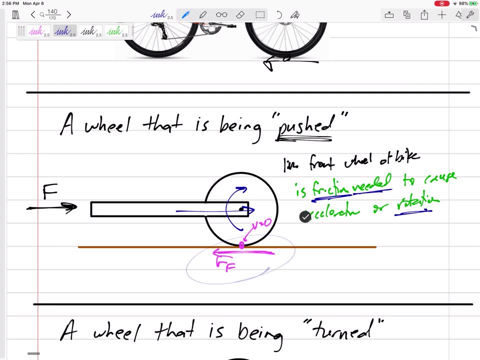 this wheel would not rotate, And I know that this wheel is rotating right- A wheel that is being pushed. it is rotating. If it's going forward, what direction is it rotating? It is rotating that way. So in this case, the force of friction will be that way, because if it wasn't there, there would. 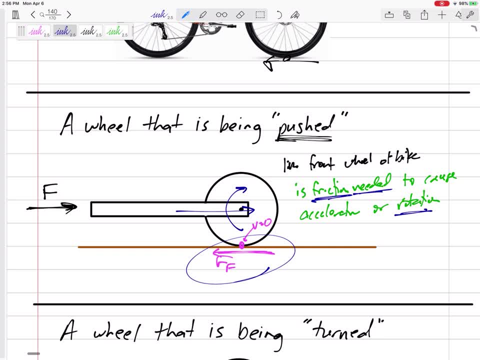 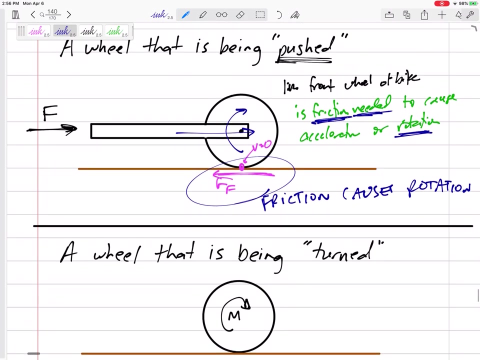 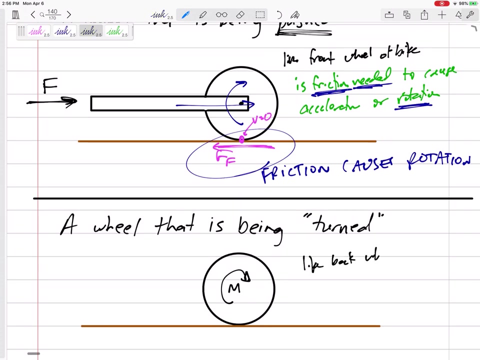 be no rotation. So in the front wheel, a wheel that's being pushed, the friction causes the rotation. Friction causes rotation. Okay, but a wheel that is being twisted- alright, a wheel that is being twisted like the back wheel of the bike when you're pedaling. 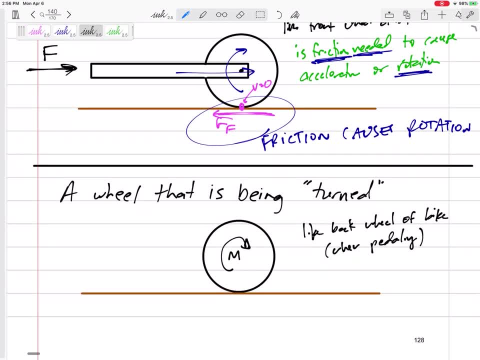 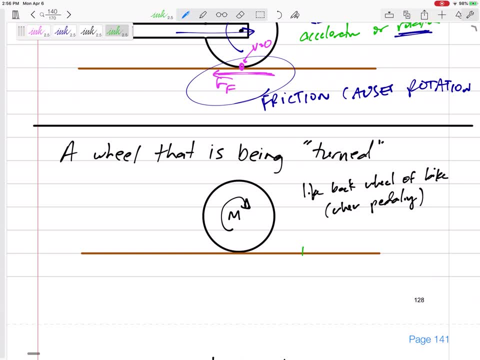 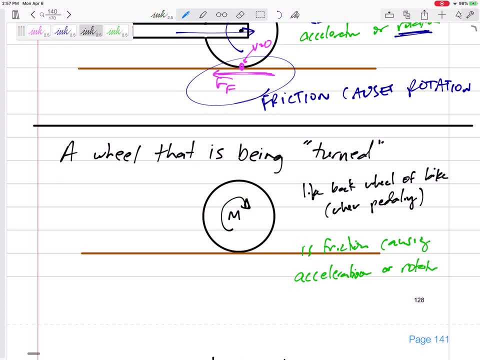 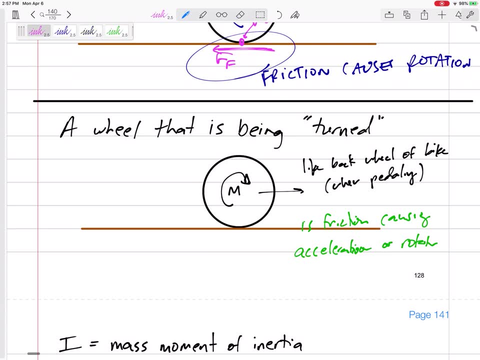 So if I give this wheel a twist, it's going to go forward. Is friction causing the acceleration or the rotation? So if I give this wheel a twist, it's going to go forward. Is friction causing the acceleration or the rotation? So if I give this wheel a twist, it's going to go forward. Is friction causing the acceleration or the rotation? 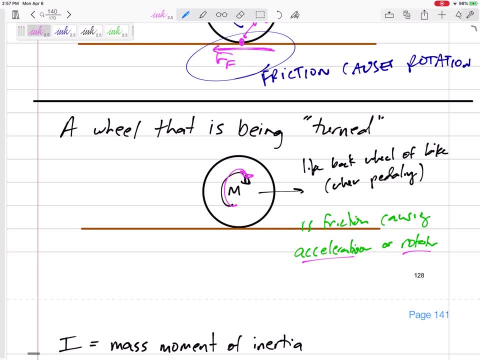 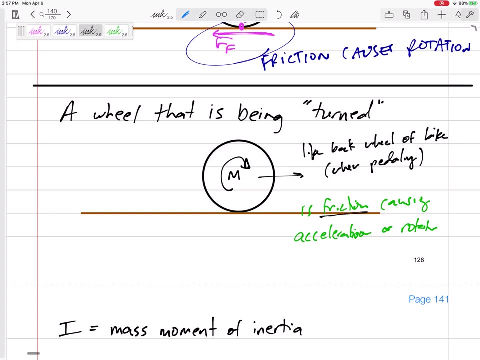 The moment is already causing the rotation right Friction. in this case, friction, is what causes it to go forward. So my force of friction would be forward right here. In this case, friction, friction is causing the rotation. no, no, no, no, sorry, Friction is causing it to move forward. In this case, friction. friction is causing the rotation- no, no, no, no, sorry. Friction is causing it to move forward, And we've got the force of friction right there. And we've got the force of friction right there. 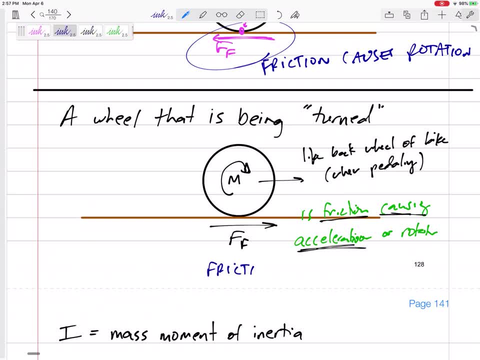 And we've got the force of friction right there. In this case, friction causes the motion forward. This is like your wheels on the car. You've got the shaft that is twisting the wheels and friction causes your car to go forwards. Friction is the force that causes your car to go forwards. 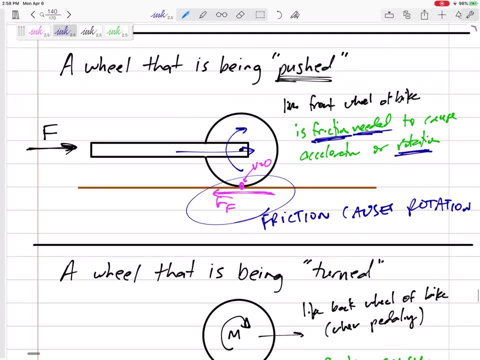 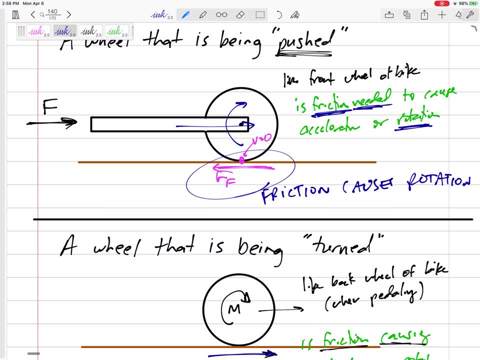 So, anyway, wheels, just ask yourself: without friction, what is friction needed? What does friction do? What's the purpose of friction for this problem, For wheels that are being pushed, friction is what's causing the rotation. So think about. I know which way it's rotating and force or friction causes that rotation. 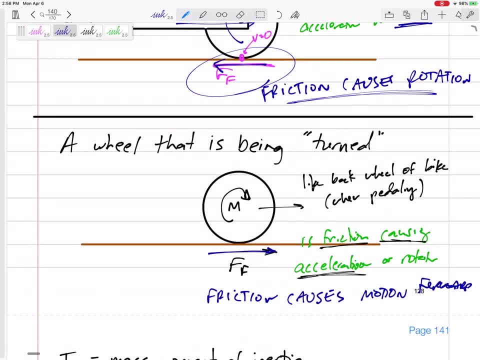 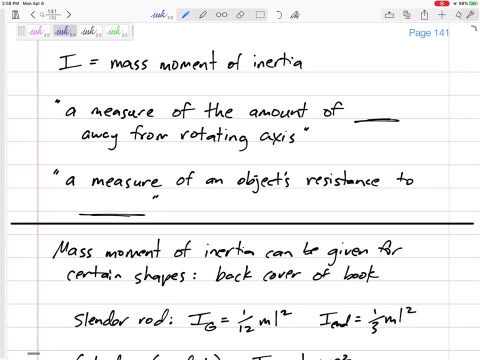 Or the friction causes the car to go forward, Or many times you will see it. you'll figure it out throughout the problem. if you don't see it already, Okay, let's talk about I mass moment of inertia. Mass moment of inertia is the measure of the amount of mass and how far it is away from the rotating axis. 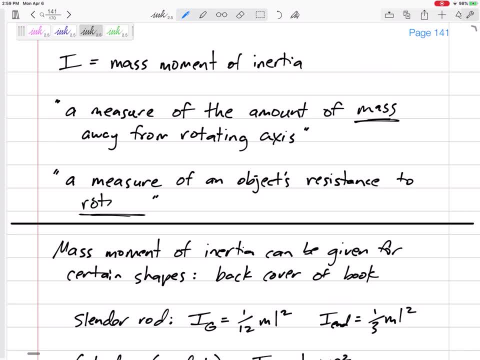 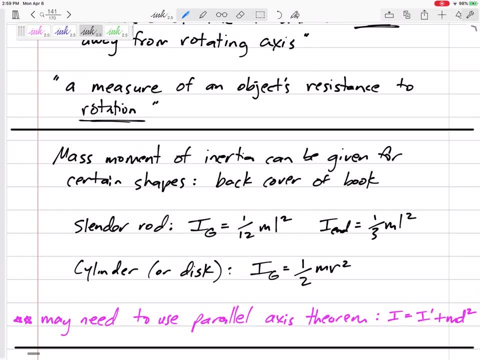 It's really a measure of an object's resistance to rotation, Measure of an object's resistance to rotation. So the moments of inertia are given Given for common shapes. we've got a slender rod. it's one-twelfth ML squared about the center of the slender rod. 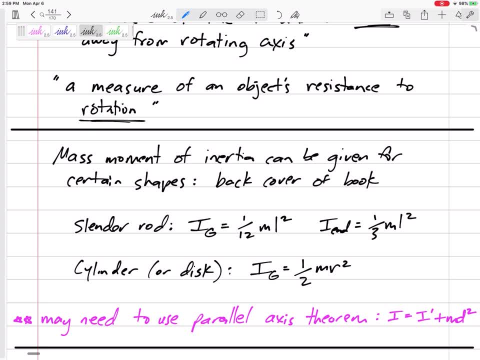 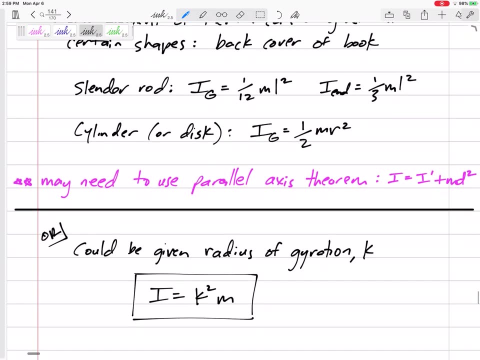 The I about the end of a slender rod is one-third ML squared. So if we were twisting a rod about its end, it would be one-third ML squared. The I about a cylinder or a uniform disc is one-half MR squared. Don't forget about the parallel axis theorem. 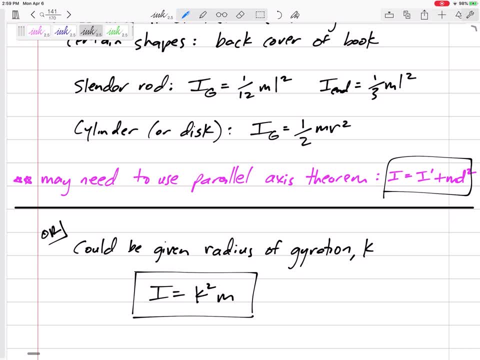 So if they give us the I about one point but we want to know the I about a different point, we would add MD squared. take the I that they give us but then add MD squared. Or they could give us the radius of gyration K. 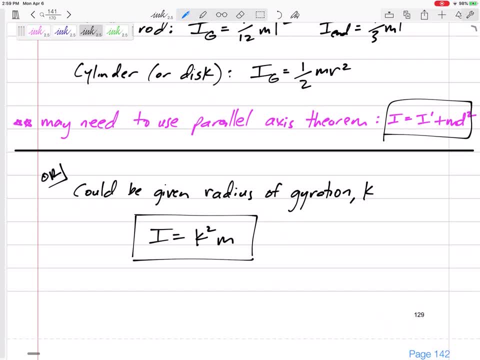 Alright, and K is a value that we can use to find I. I is equal to K squared times mass. I is equal to K squared times mass. So if they give us the K, especially if it's not a uniform disc, 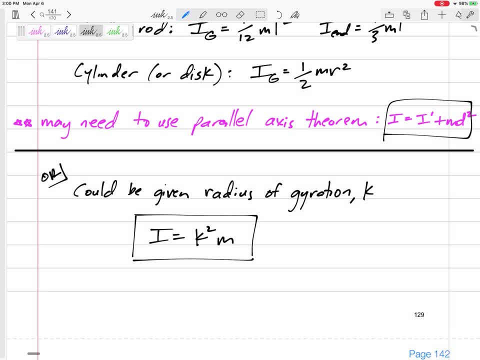 if it's not a uniform wheel, they might give us the radius of gyration and we could do K squared M to get the mass moment of inertia. I Alright. so now I said some of the moments equals I alpha. That's not exactly true. 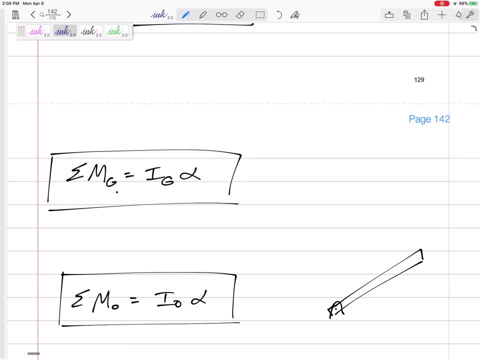 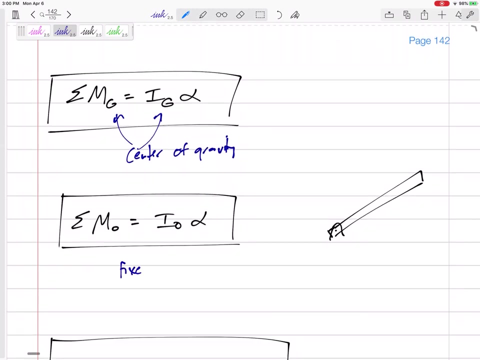 It's true if we sum the moments about the center of gravity. Alright, so yes, some of the moments about the center of gravity is equal to I about the center of gravity times alpha of that object. It's also true if I sum the moments about a fixed point. 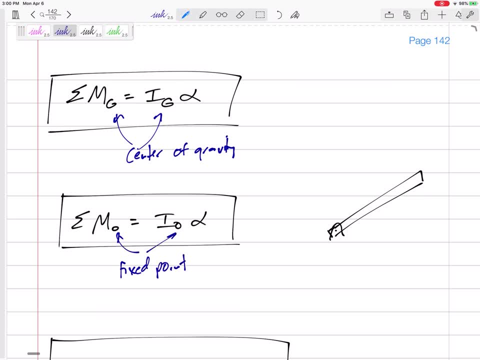 a point that is not moving. For instance, let's say we've got a link that is pinned right here at O. If I sum the moments about G, it would be equal to I- G- alpha. If I sum the moments about O, it would be equal to I about O- alpha. 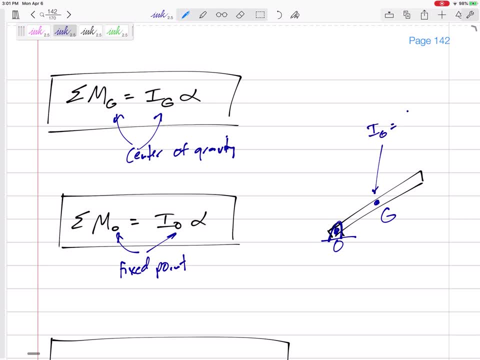 And so, for a slender rod, the I about G is one point One twelfth M L squared. So I would you know, plug in one twelfth M L squared. If I sum the moments about G, it would be equal to I, G, alpha. 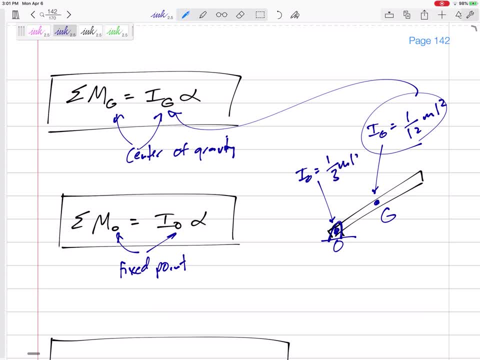 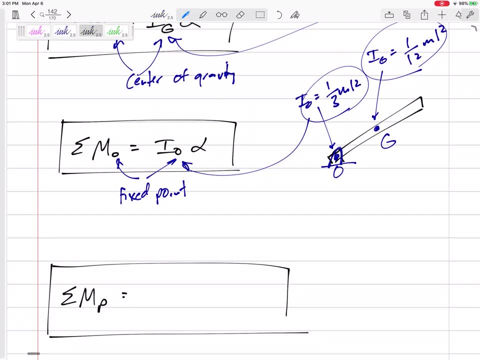 The I about the end of a slender rod is one third M L squared. So if I sum the moments about point O, it would be equal to I about point O, alpha. But if I sum the moments about a different point, P, let's call this P, a point that is not the center of gravity. 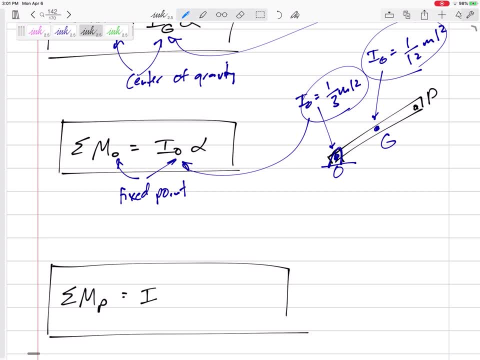 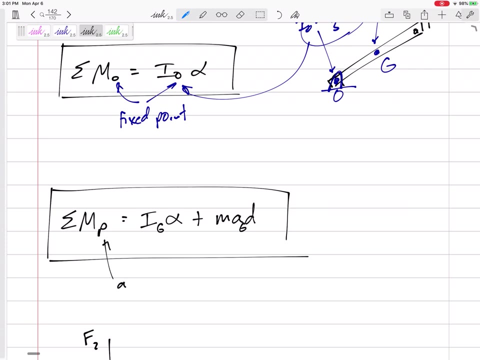 and a point that is moving, then this would be equal to I G alpha plus, and it could be minus M A D. This is the A of G. So if I sum the moments about a different point, it would be equal to I G alpha plus M A D. 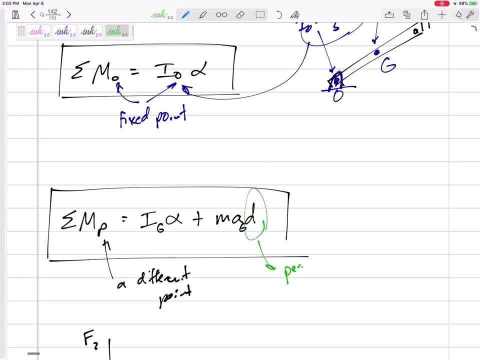 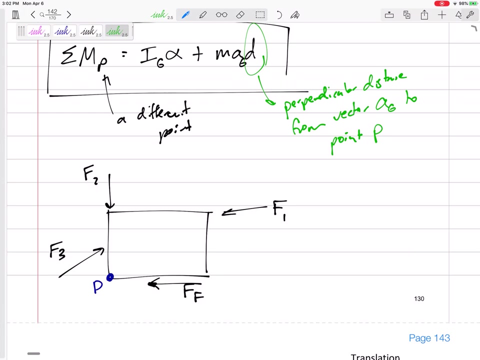 And D is the perpendicular distance from the acceleration vector, the acceleration of G vector to point P. Perpendicular distance from the acceleration vector to point P, For instance, for instance. let's look at this one. Let's look at this one. 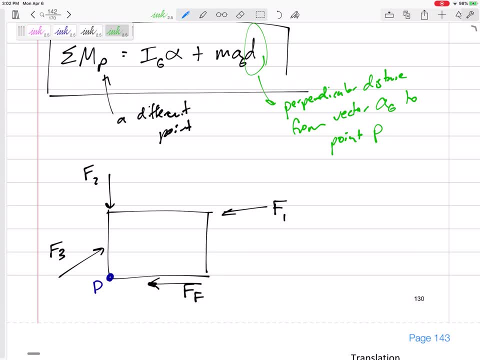 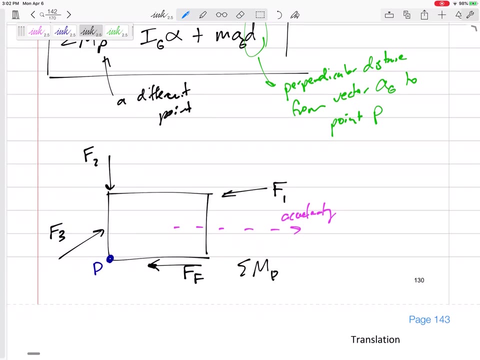 Let's say we have a box and it has as high as all these forces on here. Let's say it is accelerating to the right. Maybe this is sliding on the ground. It's accelerating to the right If I wanted to- and there may be occasions where I will want to- 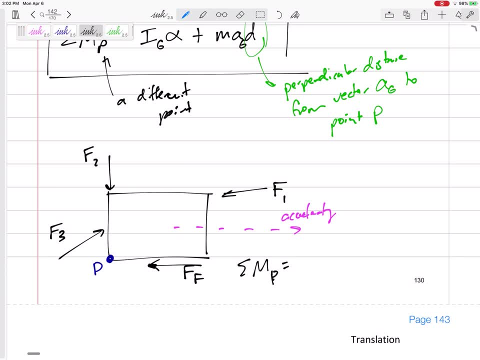 if I wanted to sum the moments about point P, it would be equal to I G alpha. Now if it is just sliding, that alpha could still be zero. It could be zero if there is no rotation, If it is just sliding across the ground. 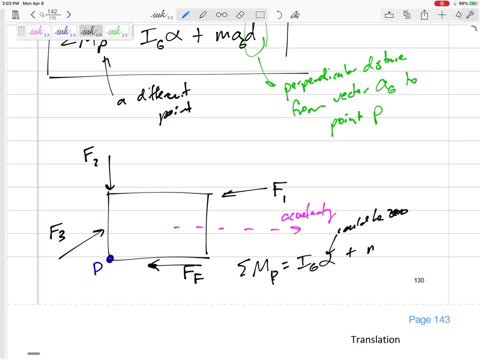 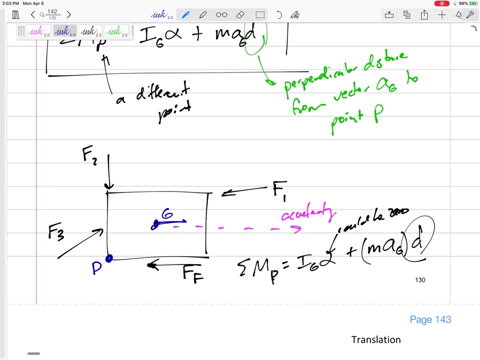 it could be zero, But I need this M, A, D term. And what is D? D is the perpendicular distance from the vector, from the acceleration vector. So let's say this is point G, My acceleration vector is right there. The perpendicular distance from there to point P: 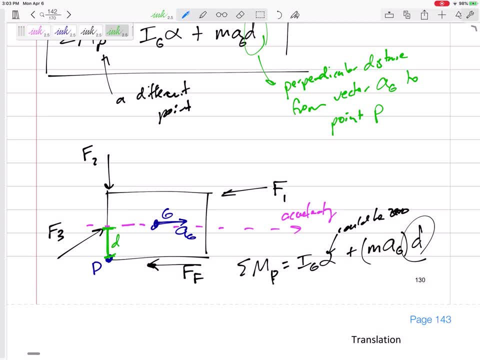 would be this distance right there, That distance right there. Let's say this is three inches, It would be that three inches right here, It would not be that five inches. The distance is going to be perpendicular to the acceleration vector. Perpendicular to the acceleration vector. 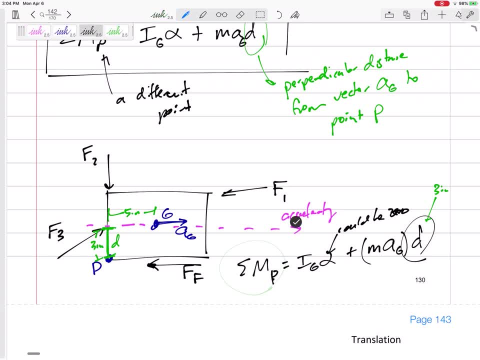 And one last thing: We are summing the moments about P. If we have been summing the moments about P counterclockwise positive, then this M A vector and this D- it is almost like this creates a moment. It doesn't really. 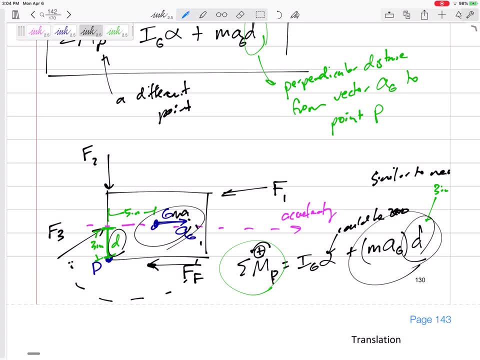 Similar to a moment, Alright, And if we have been summing everything counterclockwise, this acceleration about point P, it is almost like a negative moment, And so in this case we would have a negative M A D. So do that M A D as if the M A D was a moment. 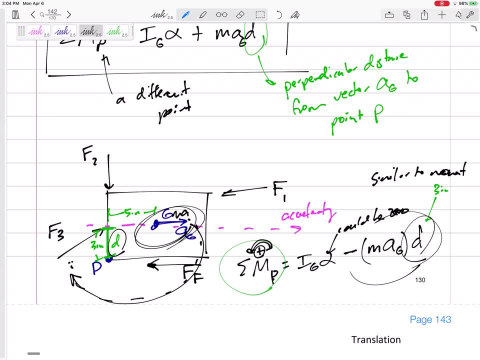 And we have been summing the moments. And so let's be consistent: If we have been summing the moments counterclockwise, if this alpha counterclockwise positive, then this needs to be counterclockwise positive, And in this scenario, 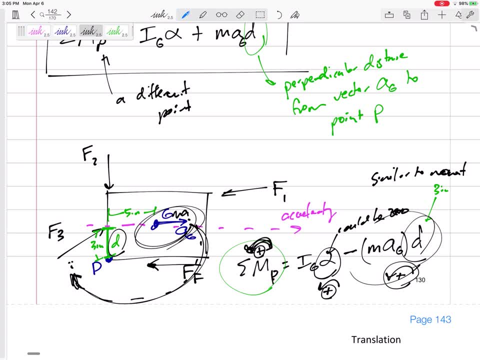 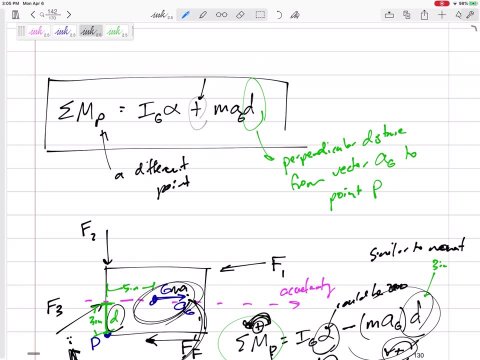 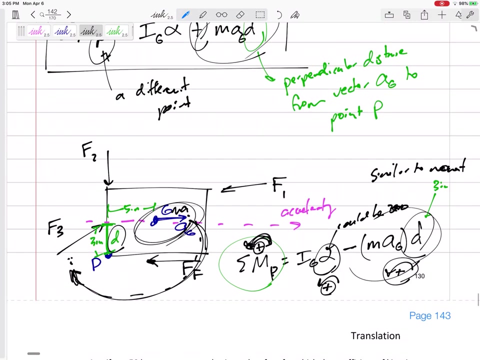 that would be a clockwise M A D, making it a negative minus M A D. So this might be plus, could be negative, Depending on that M A D. does that create a positive moment about P or a negative moment about P? Okay, 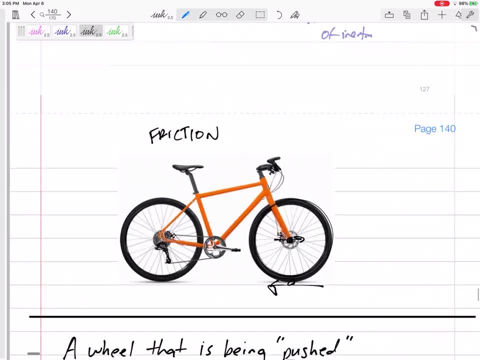 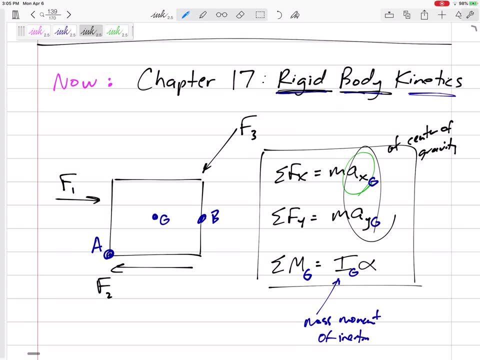 But let me reiterate, Circle back. We are still going to sum the forces in X equals M A X. Sum the forces in Y equals M A Y. Now we are going to sum the moments, And if we sum the moments about G, 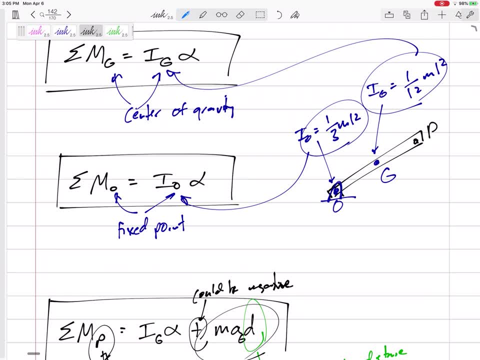 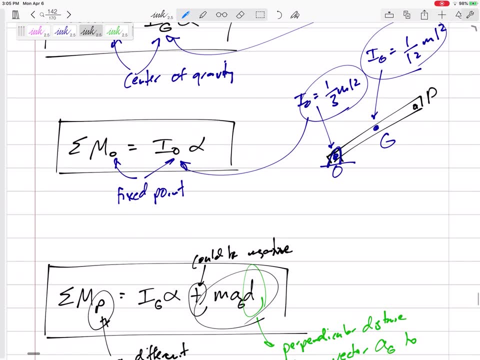 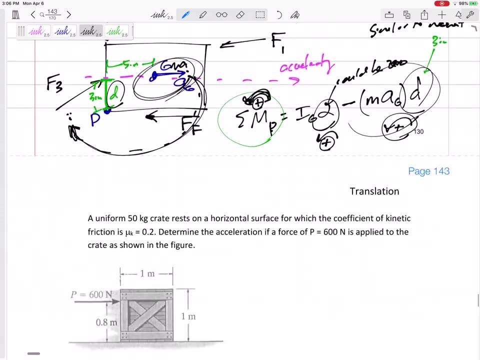 it is I G alpha. If we sum the moments about a fixed point, it is I about the fixed point, alpha. If we sum the moments about a point P, it is I G alpha, plus, maybe minus M A D. So we are going to start with some translations. 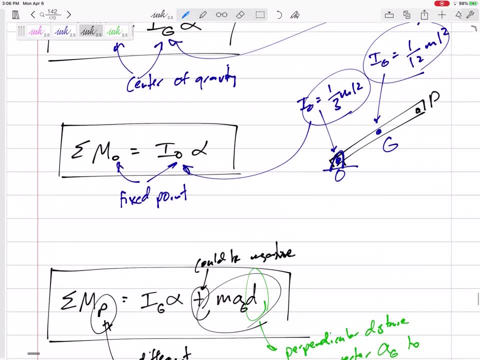 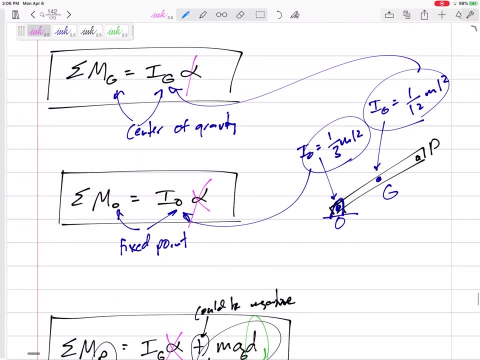 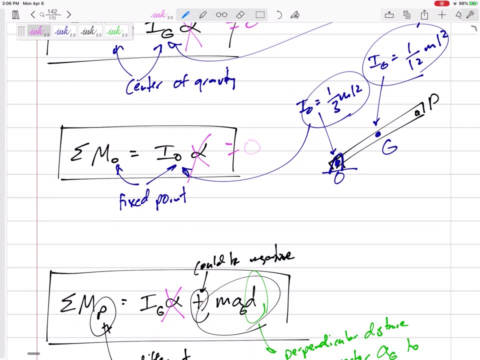 Okay, And in translation. in translation alpha is zero, So some of the moments would be zero in translation. Some of the moments about a fixed point would be zero in translation. But if I sum the moments about point P, here is the important thing. 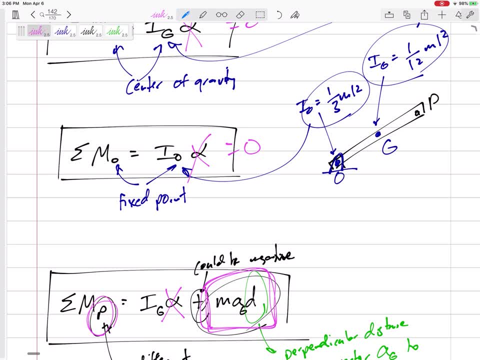 I might. it might not be equal to zero, even if it is in translation. Does that make sense? Translation might still be. some of the moments might be equal to something if I sum my moments about a different point: P, Okay, Okay. 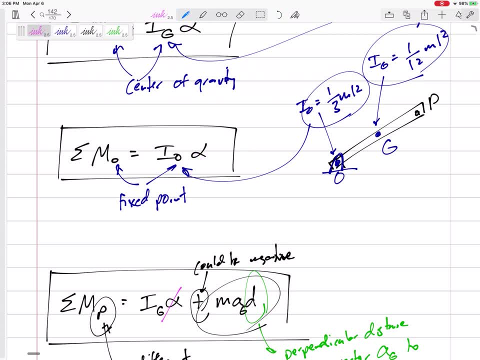 So next thing we will do is just start with some translation problems.